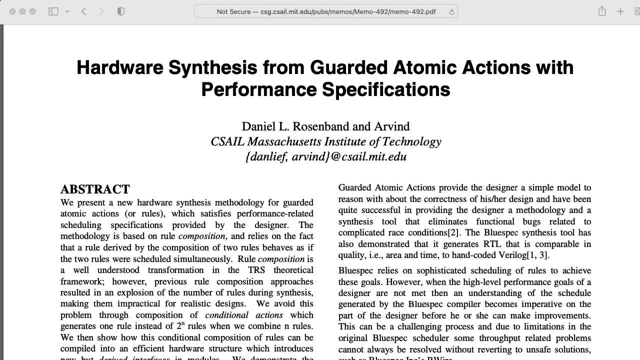 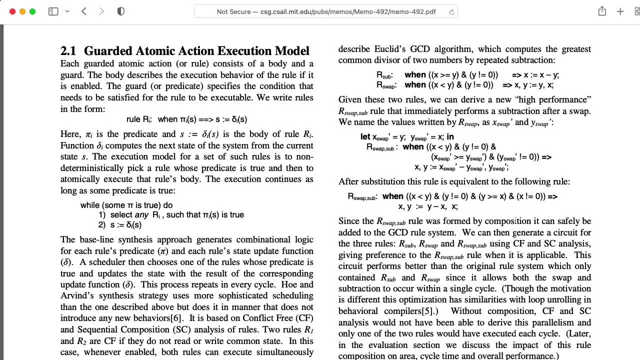 a language called BlueSpec. BlueSpec is apparently built around the idea of guarded atomic actions, Whatever those are. I haven't really looked into this in detail yet. BlueSpec was formulated by Arvind, a computer scientist at MIT who is so incredibly awesome. 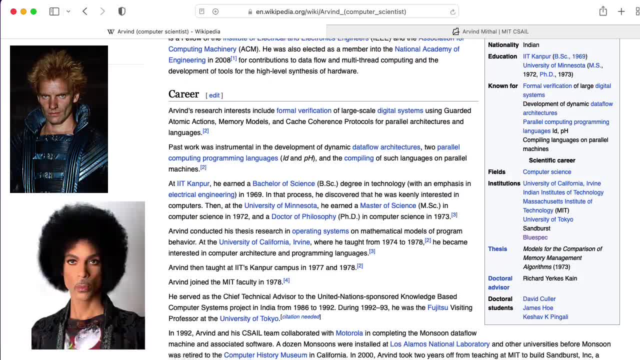 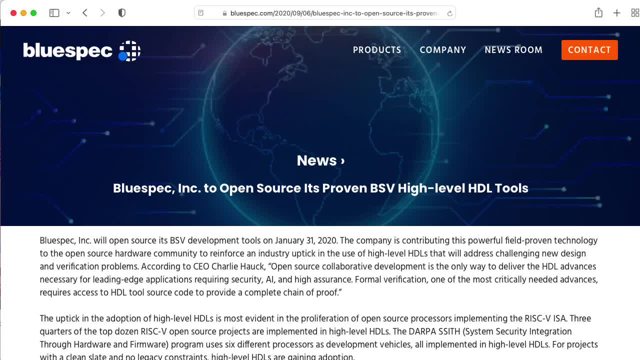 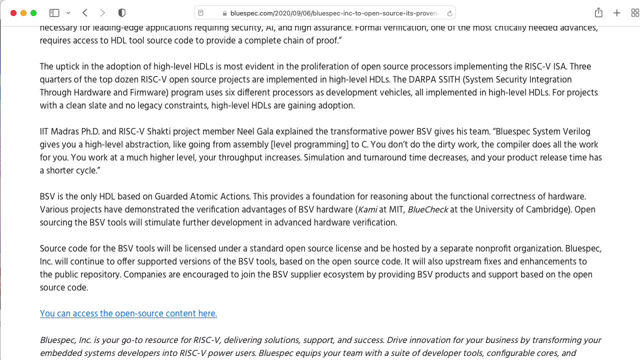 that he just goes by one name, like Sting or Prince BlueSpec was once a proprietary and probably pretty expensive language. It was open-sourced in 2020, which is a good thing, because nowadays, keeping your language proprietary is basically saying that you want your language to die. Now it's a little confusing because if you go to the 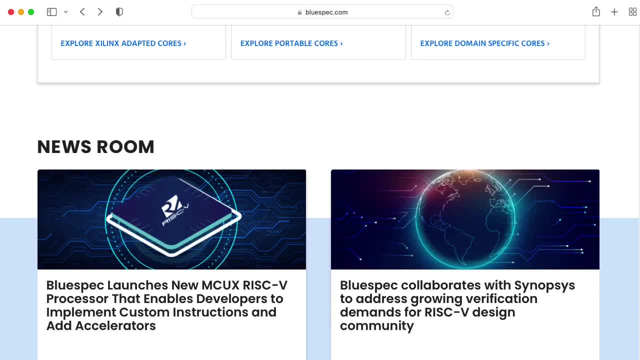 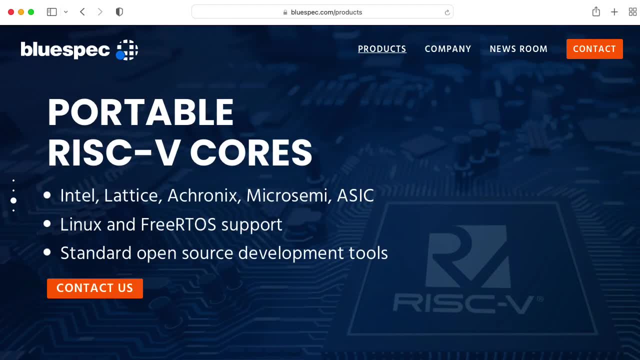 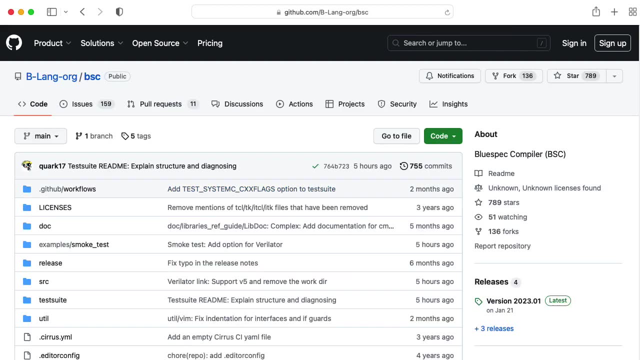 BlueSpec website. it doesn't look like there's anything here about their languages. There's just a bunch of stuff about RISC-V and FBGAs. You have to find Beelang on GitHub and go to the BSC repository. Now there's actually two versions of the BlueSpec language. One is BlueSpec System. 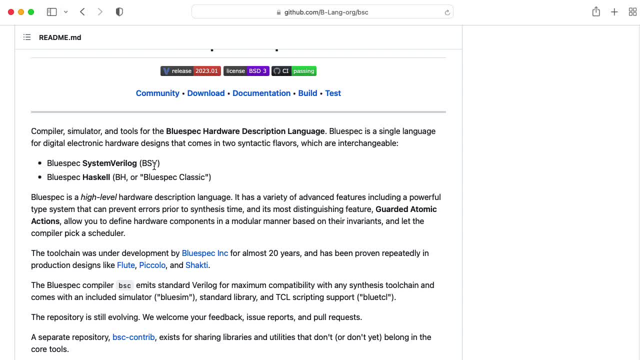 Verilog BSV, which I think is the most common version of the BlueSpec language. The other one is a compromise to help get people familiar with Verilog into BlueSpec. but I think the soul of BlueSpec is in BlueSpec Haskell. Haskell is a functional programming language that's popular. 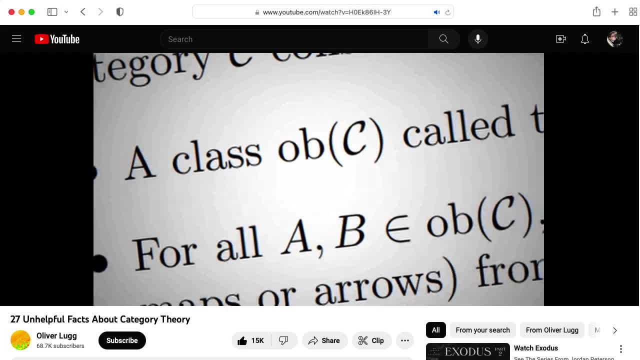 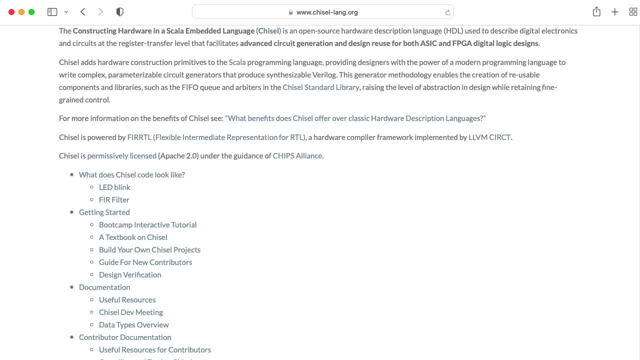 with computer science nerds, particularly people who talk about category theory and weird stuff like that. Another open-source hardware description language that's getting a lot of attention is Chisel, which intends to bring some Scala action to the HDL party. I should note that. 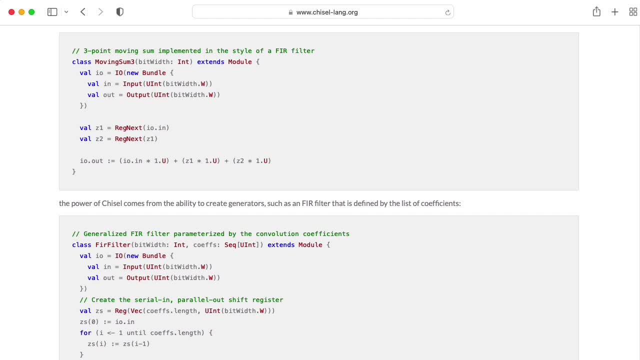 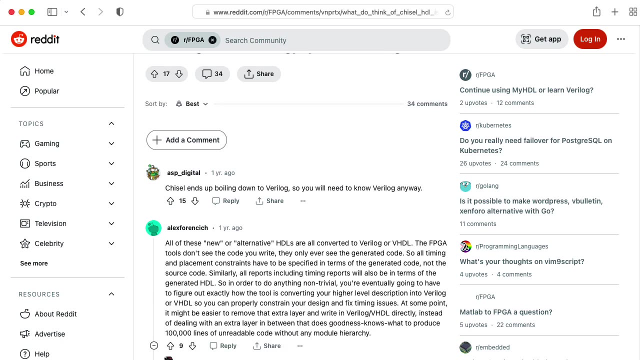 both BlueSpec and Chisel are not the same language. They're not the same language. They're the same style, down to Verilog. so you kind of have to learn Verilog regardless. Anyway, I want to hear from you: Have you used Chisel or BlueSpec? What did you think about them? 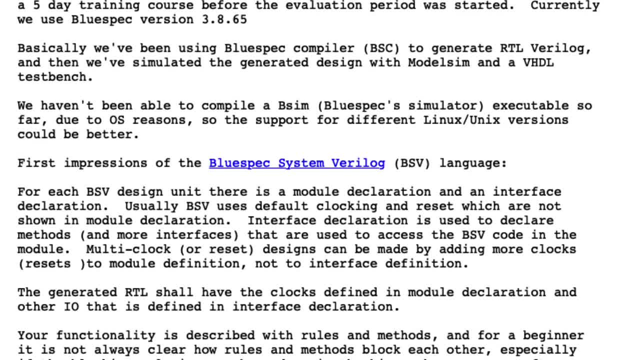 Have you used another alternative to Verilog and VHDL that I should have on my radar screen?